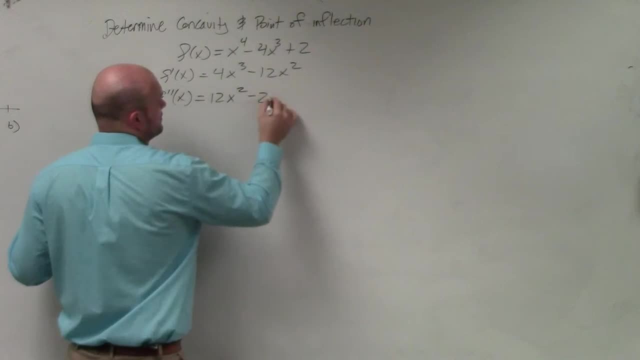 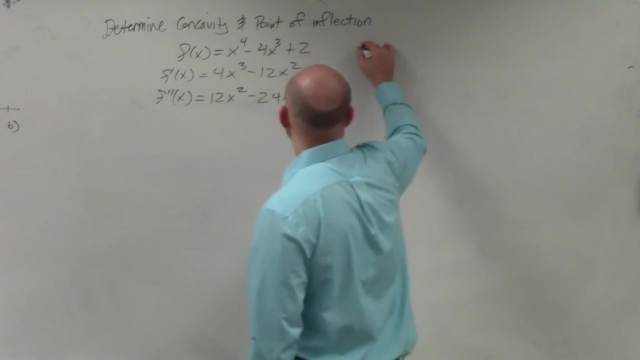 take the second derivative, Then we need to identify our possible points of inflection. So we set our second derivative equal to 0. And now what we need to do is obviously solve for x. So we're going to use some factoring techniques. I can factor out a 12x If I factor. 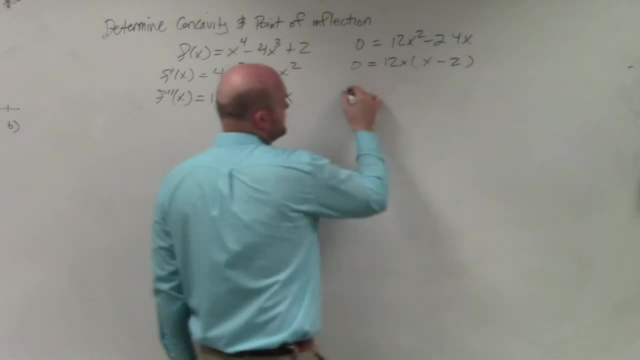 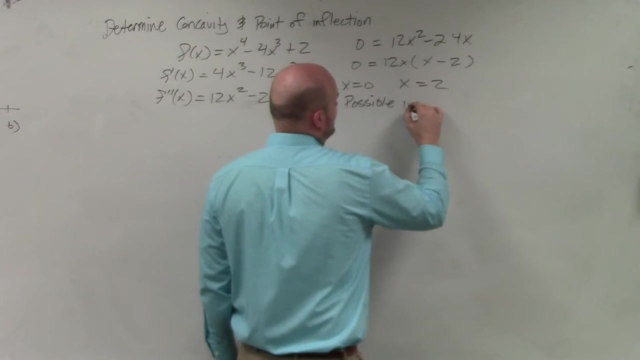 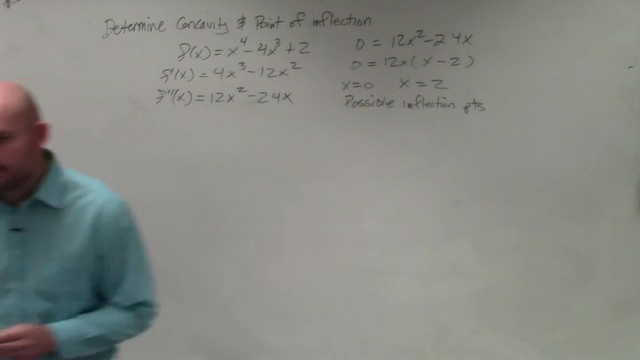 out a 12x, I get x minus 2.. So therefore I can say x equals 0 and x equals 2 are possible inflection points or possible points of inflection. OK, now we need to go and take a look at our intervals. So I'll say from negative infinity. 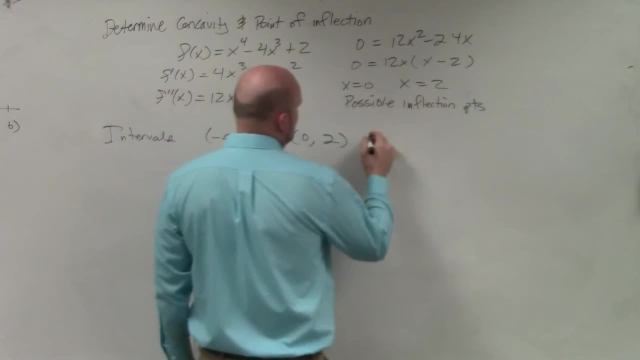 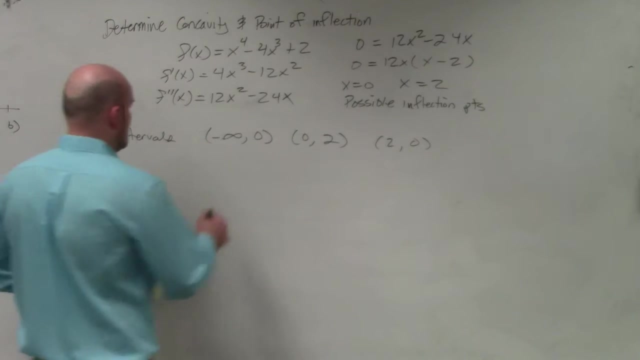 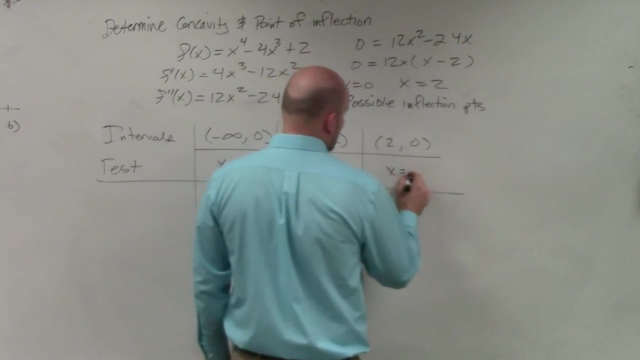 to 0,, 0 to 2, and 2 to 0.. I'll choose some test points. I'll test: x equals negative 1,, x equals 1, and x equals 3.. Again, all I need to do is: 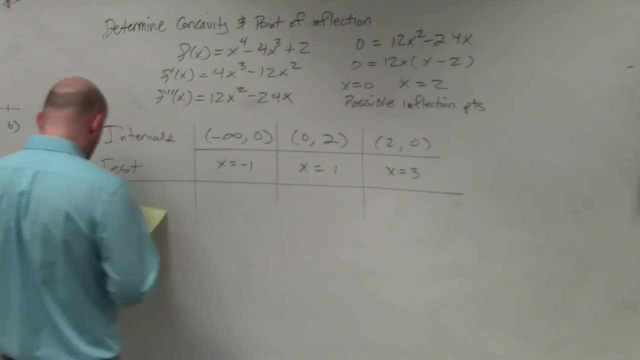 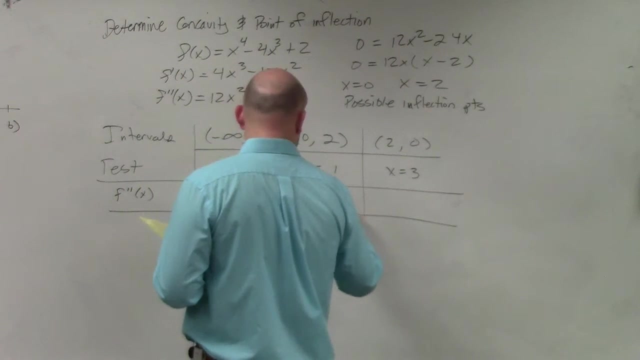 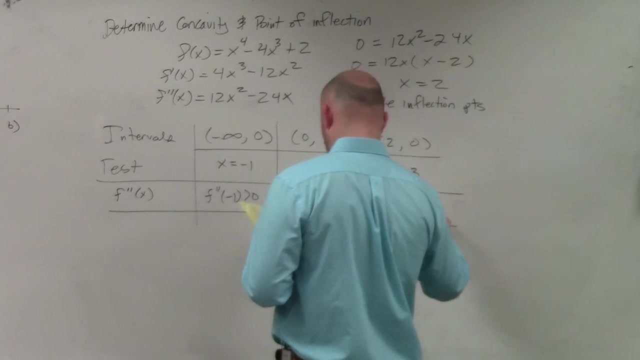 plug these into my second derivative to determine if they're going to be positive or negative. Where did I put that? OK, so, as what you guys can see is by using these tests- and again I'm just doing the math in my head- 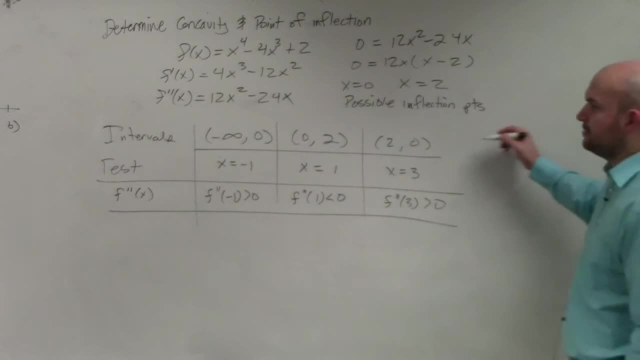 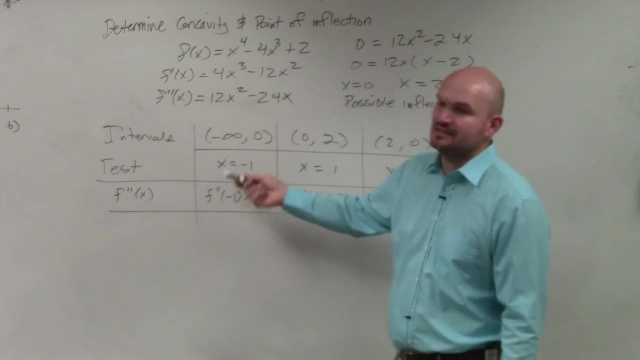 For you guys. I know I could possibly work all of these out, But to save myself some time, I'm not going to evaluate. I notice that when squaring that a negative times a negative, that's going to be a positive. 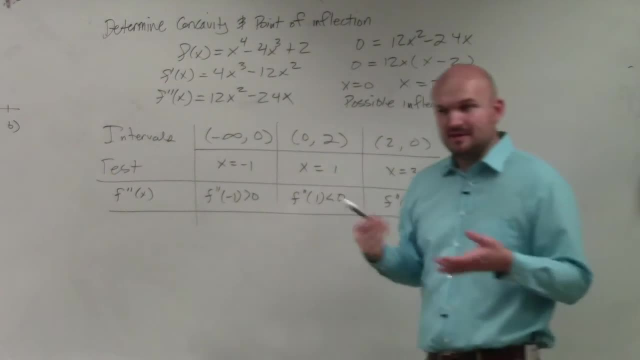 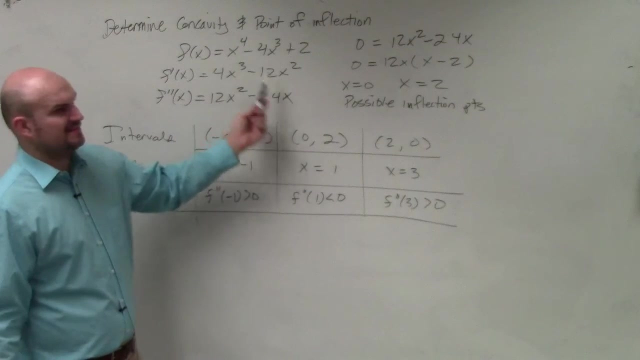 And again, I don't even need to have the right value all the time. Sometimes you're going to get points where you might not be able to do them in your head. But if you think about this, if I have a negative number, you square it, That becomes positive, Negative. 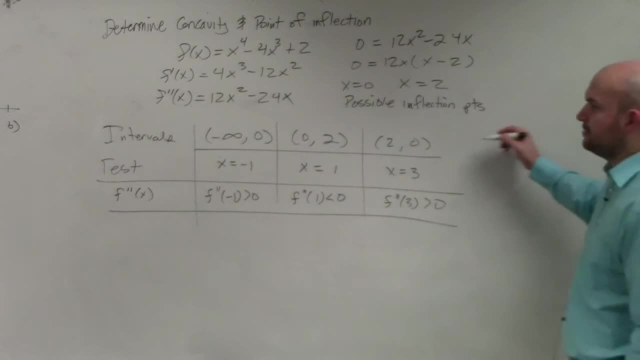 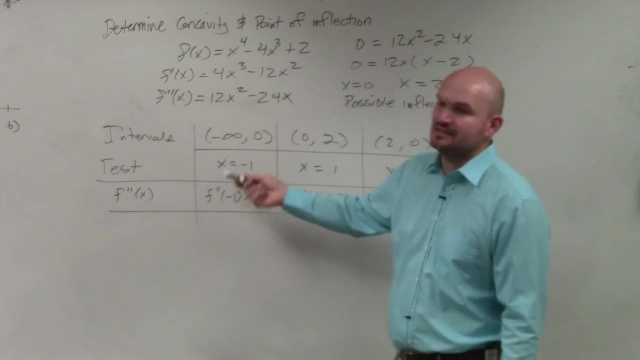 For you guys. I know I could possibly work all of these out, But to save myself some time, I'm not going to evaluate. I notice that when squaring that a negative times a negative, that's going to be a positive. 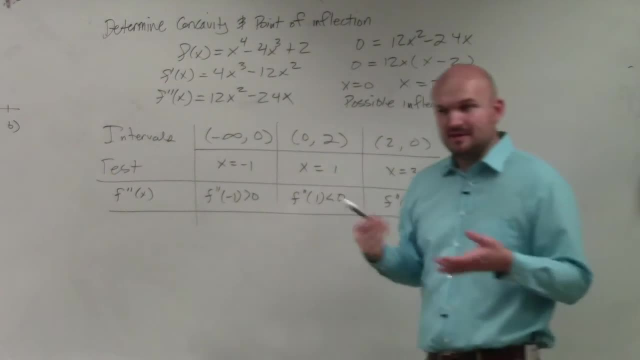 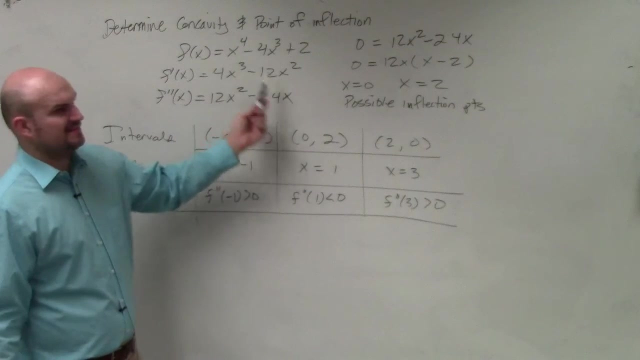 And again, I don't even need to have the right value all the time. Sometimes you're going to get points where you might not be able to do them in your head. But if you think about this, if I have a negative number, you square it, That becomes positive, Negative. 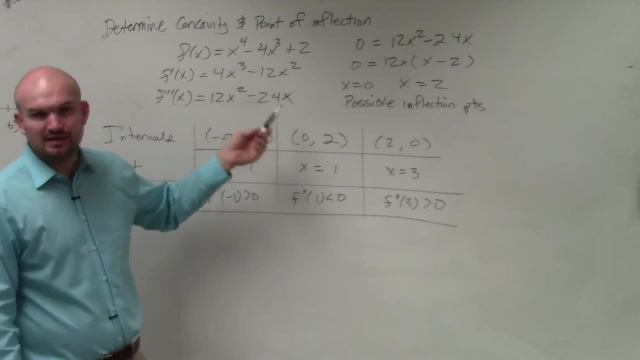 times a negative is positive. It doesn't matter really what negative number I put in here, It's always going to be positive, Right, And so just using some of these, OK, So some of that kind of thinking, Now obviously the one you'd want to just double check, make. 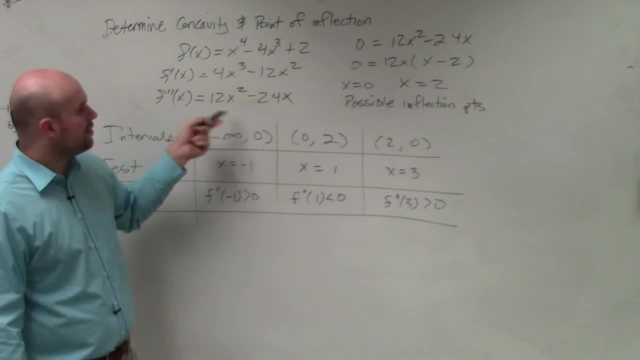 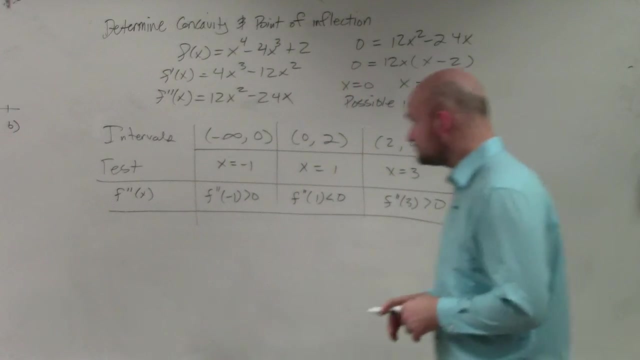 sure it's negative, And then you see 3. That, really, the 9 times 12, is going to be much larger than 24 times 3.. So that's how that ends up being back into the negative. So therefore, then we get to our last. one is the conclusion. 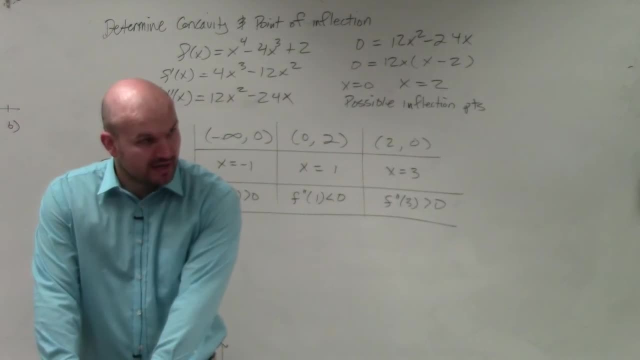 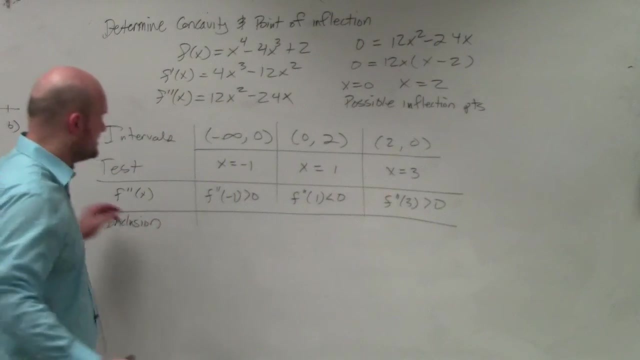 And then, ladies and gentlemen, we get into our writing portion of it, Right? So I'm going to say what the writing portion is, But to save us a little bit of time, I'm just going to write if it's concave down or up, But basically, you'd say, since f double prime negative 1 is, 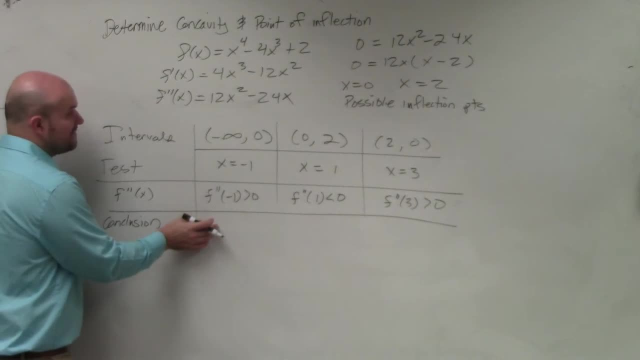 greater than 0, we could say that f of x is concave up on the interval negative infinity to 0,. right Here you could say: since f, double prime of 1 is less than 0, our f of x is going to be concave down on the interval 0 to 2.. That's what you'd want to write all. 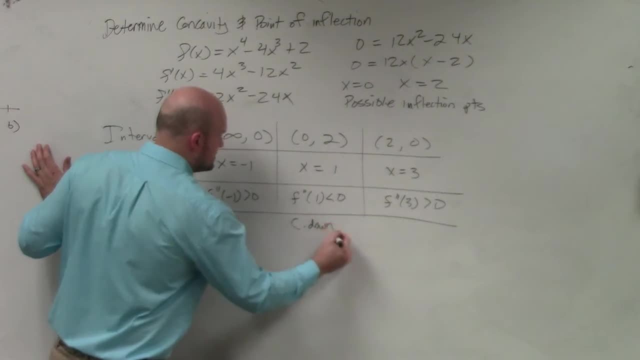 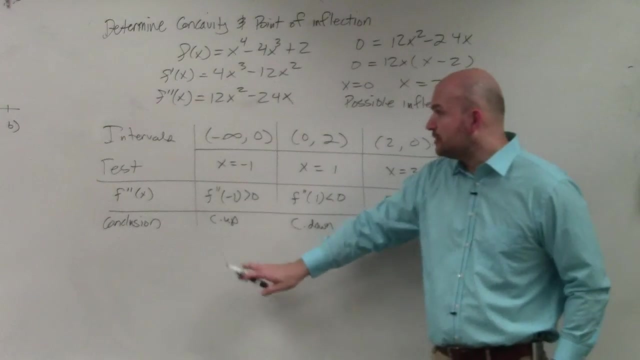 the way out, But I'm just going to save myself Some space. And then this one is concave up. And then, last but not least, ladies and gentlemen, we notice that it goes from concave up to concave down, concave down to concave up. So we could write two statements, because 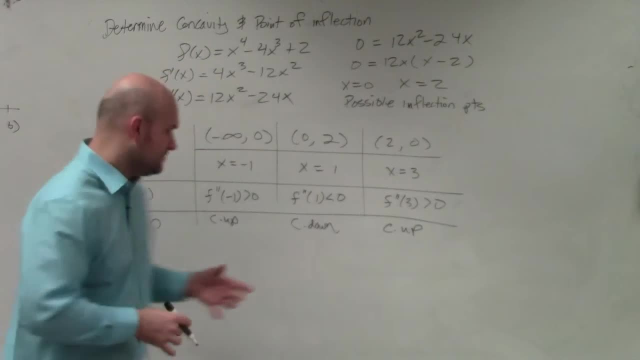 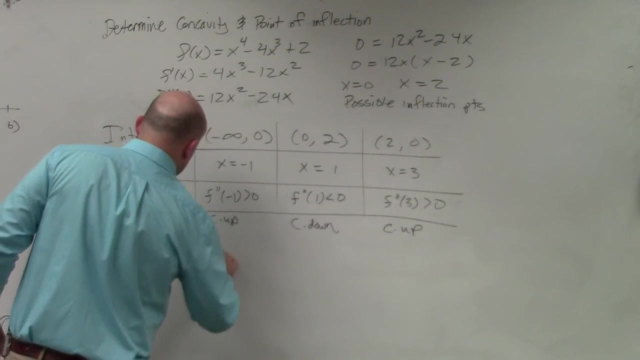 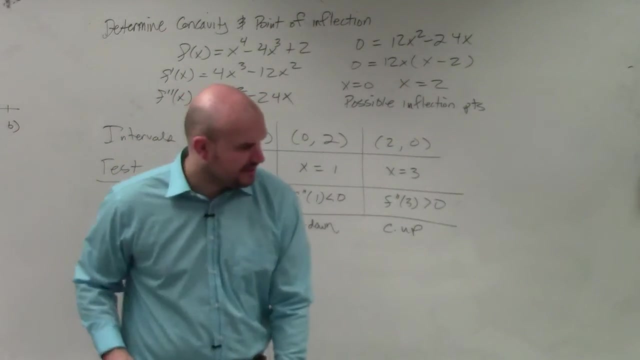 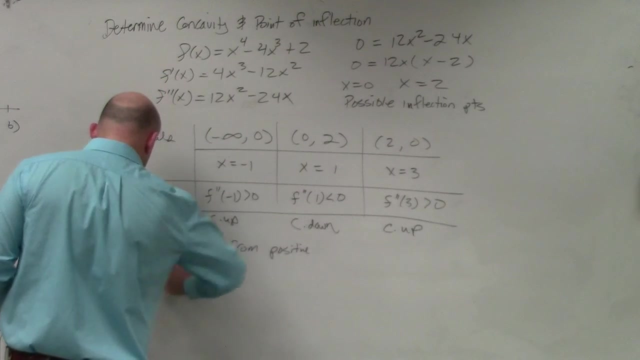 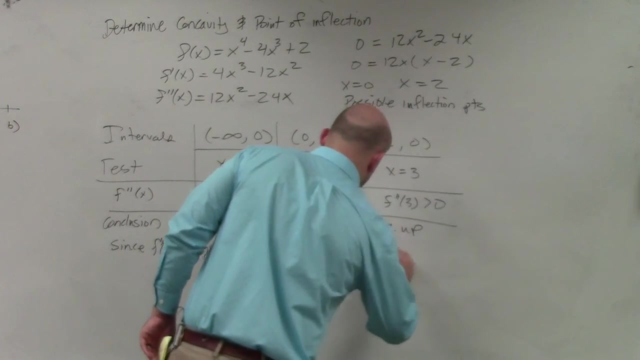 we don't want to just say it changes. We want to say what it's changing from. So we could say: since from 0 to 0.. Actually, how did I write the f double prime? You got this, sir, Yeah. 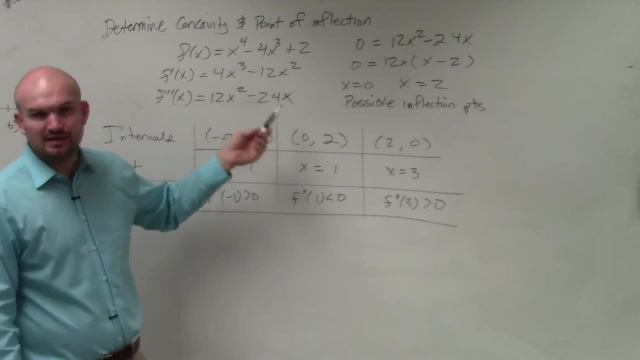 times a negative is positive. It doesn't matter really what negative number I put in here, It's always going to be positive, Right, And so just using some of these, OK, So some of that kind of thinking, Now obviously the one you'd want to just double check, make. 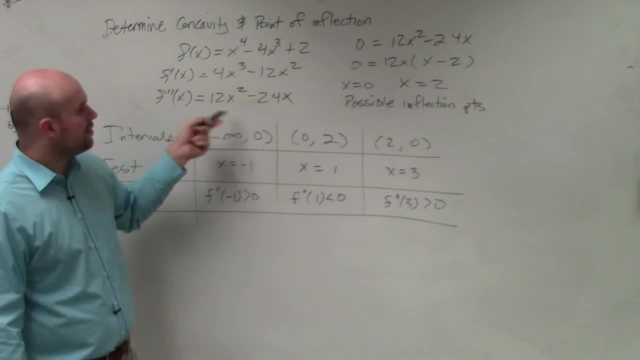 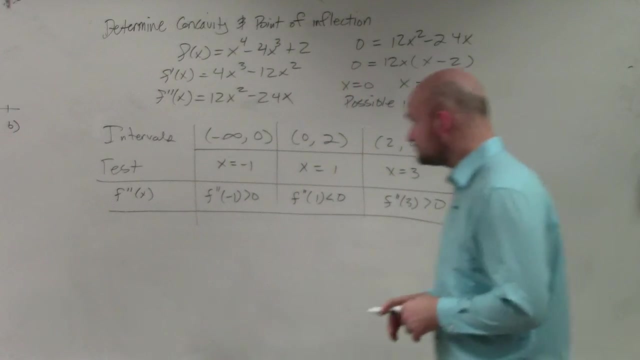 sure it's negative, And then you see 3. That, really, the 9 times 12, is going to be much larger than 24 times 3.. So that's how that ends up being back into the negative. So therefore, then we get to our last. one is the conclusion. 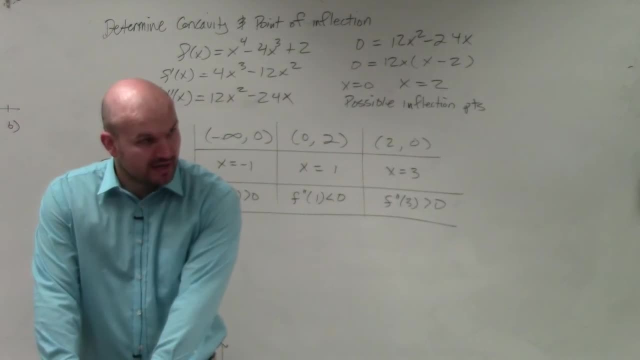 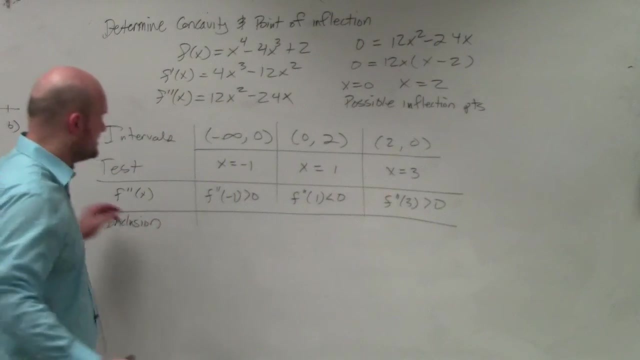 And then, ladies and gentlemen, we get into our writing portion of it, Right? So I'm going to say what the writing portion is, But to save us a little bit of time, I'm just going to write if it's concave down or up, But basically, you'd say, since f double prime negative 1 is, 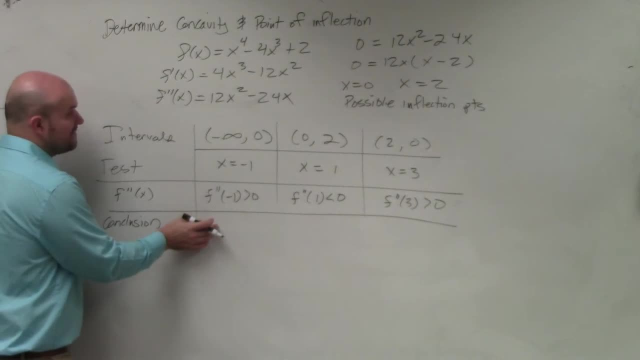 greater than 0, we could say that f of x is concave up on the interval negative infinity to 0,. right Here you could say: since f, double prime of 1 is less than 0, our f of x is going to be concave down on the interval 0 to 2.. That's what you'd want to write all. 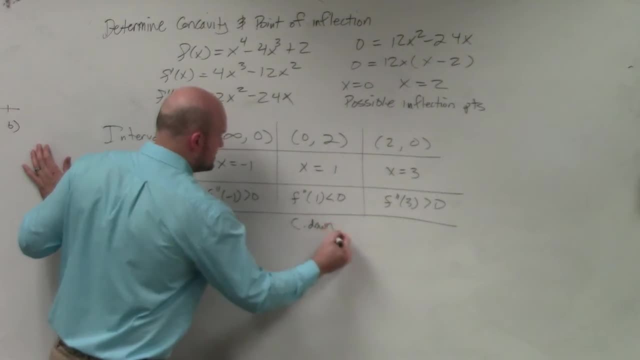 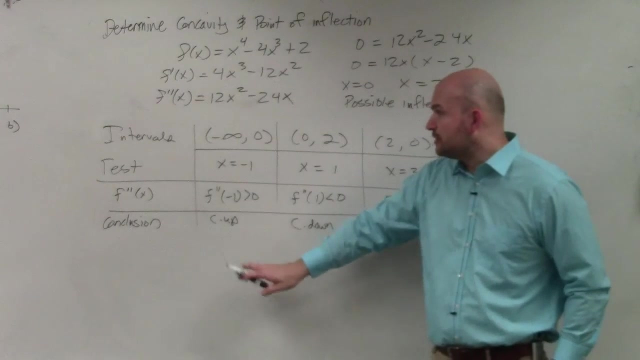 the way out, But I'm just going to save myself Some space. And then this one is concave up, OK. And then, last but not least, ladies and gentlemen, we notice that it goes from concave up to concave down, concave down to concave up. So we could write two statements, because we 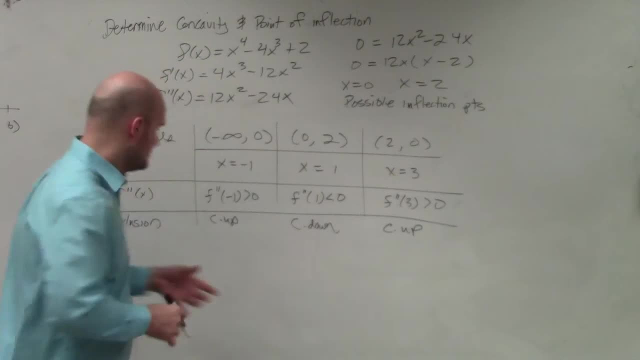 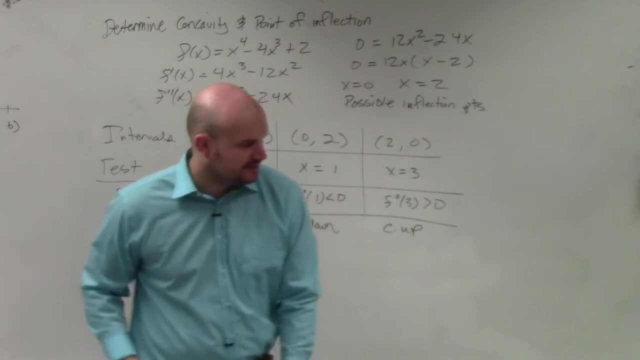 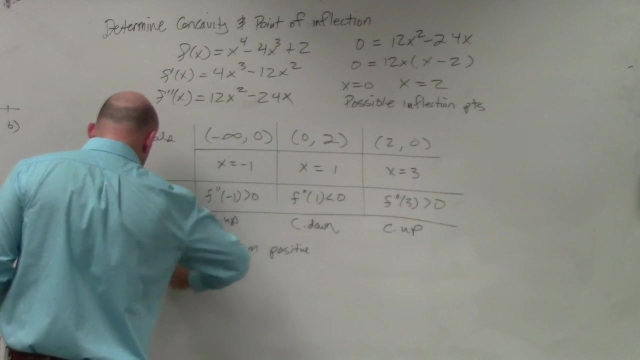 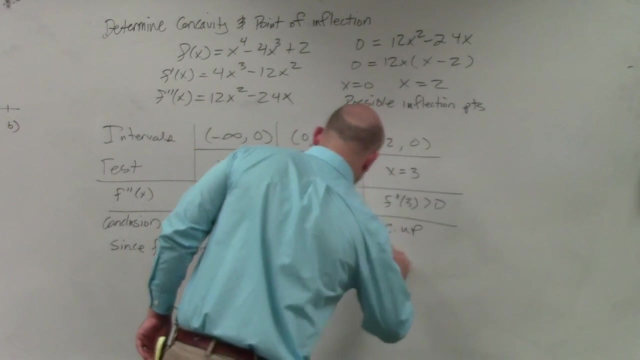 don't want to just say it changes. We want to say what it's changing from. So we could say since from 0 to 0.. Actually, how did I write the f double prime? You got this, sir, Yeah. 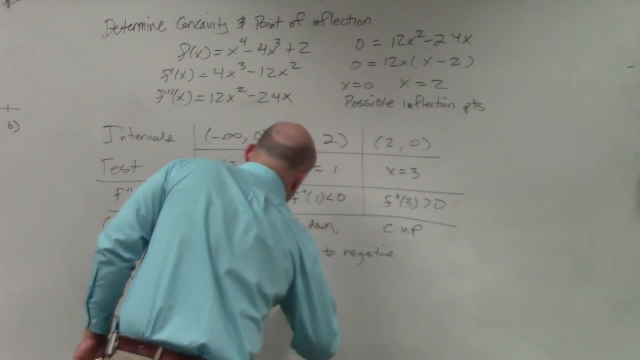 OK. So make sure when we're labeling our points of inflection we want to just say, we want to make sure that we are describing how it's a point of inflection, not just saying, since f double prime is changing signs, it's a point of inflection. go the extra step and say: